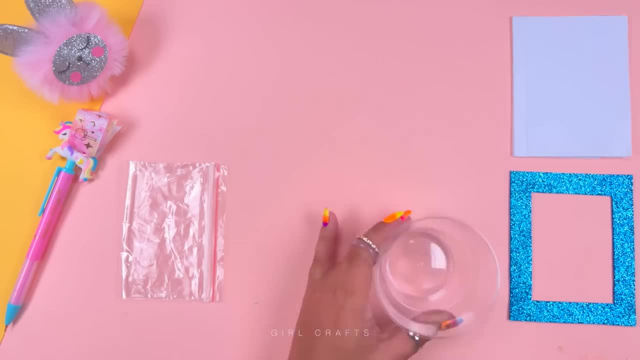 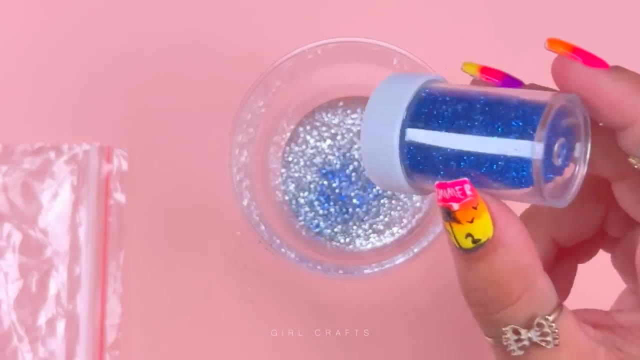 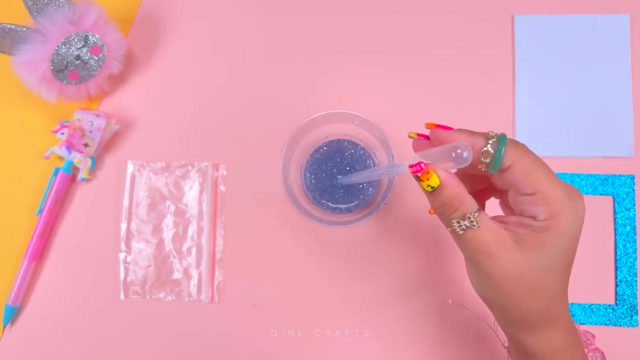 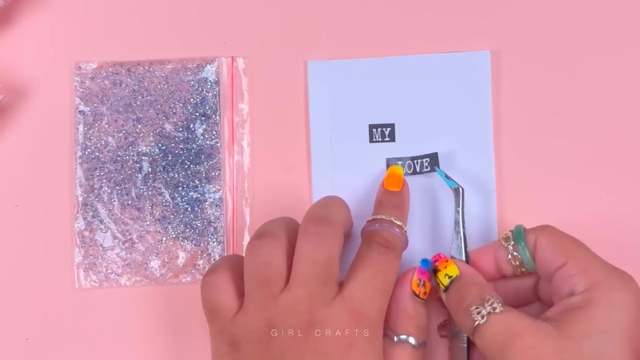 If I'll dance with the lights on, If you're gonna be moving on solo, Wait a second, cause they're playing the best song. I'll be there. if you reach out to me, Reach out to me, Reach out to me. 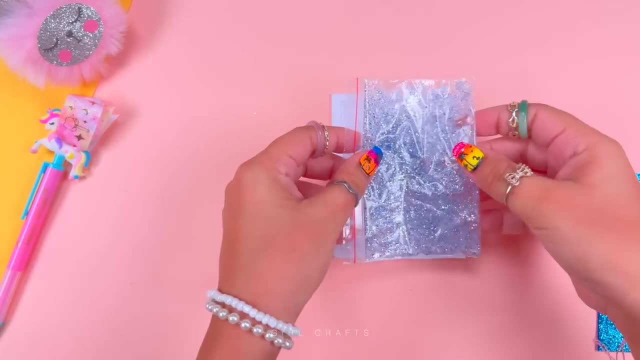 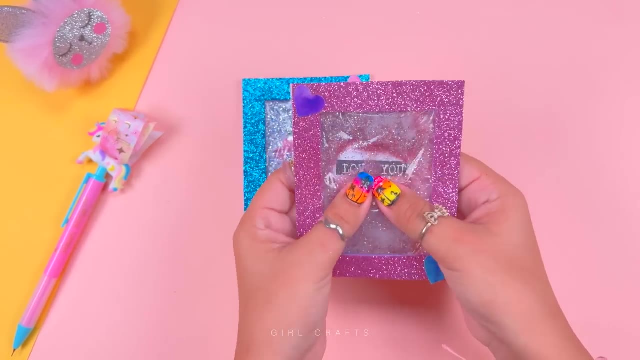 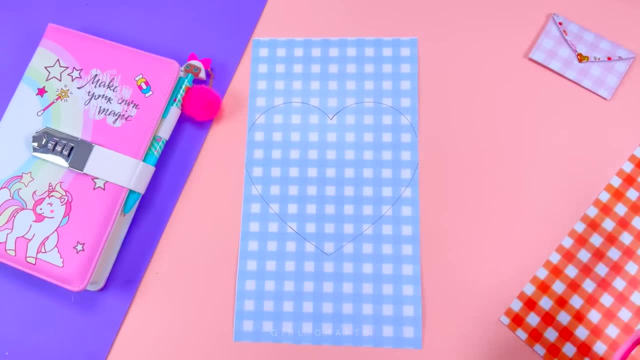 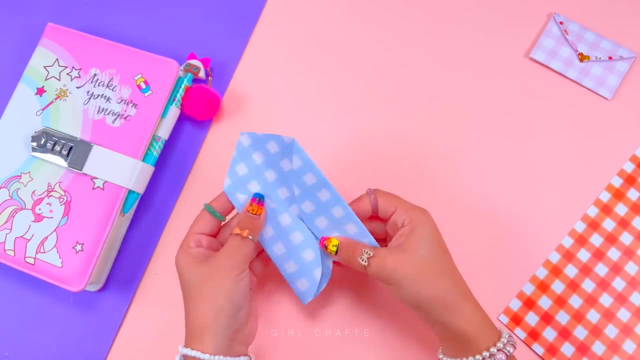 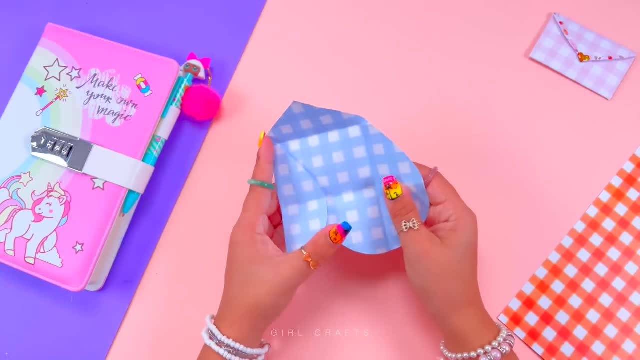 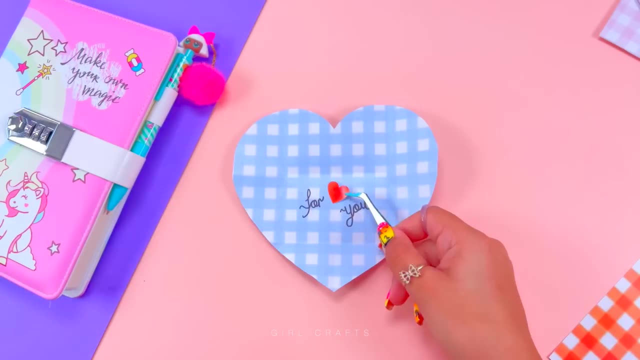 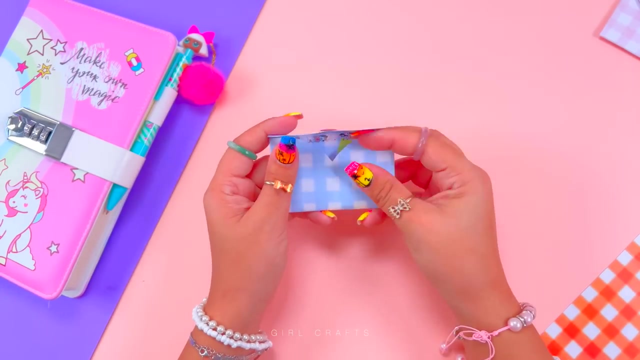 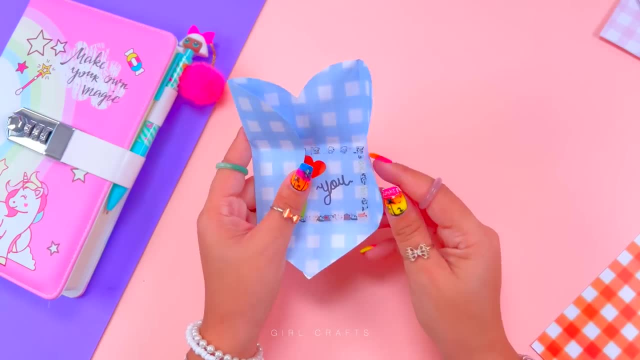 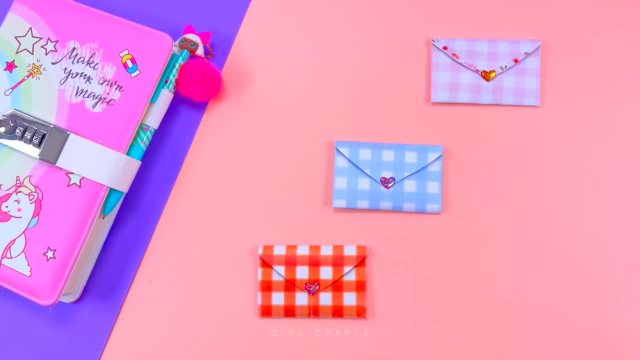 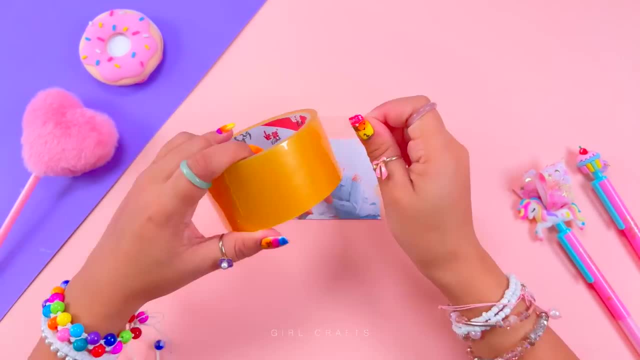 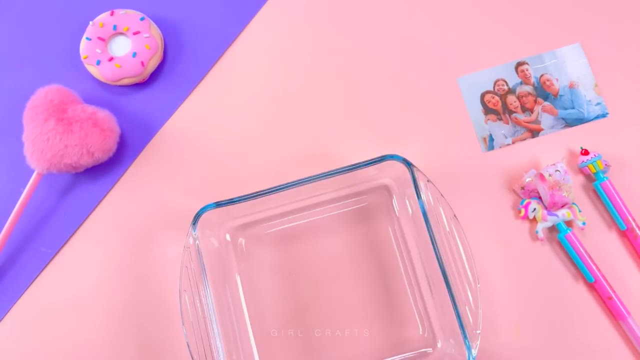 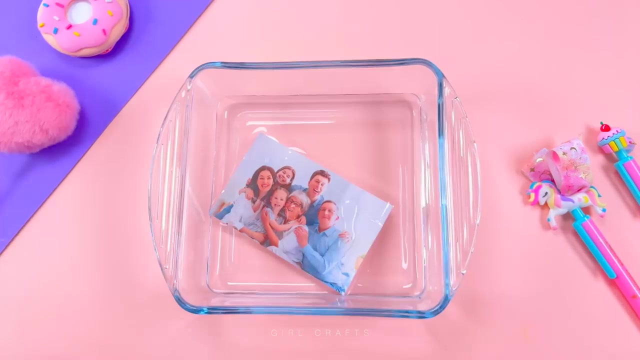 ZE, ZE, ZE, ZE, ZE, ZE. I get too drunk and too scared and lie to you. If only you knew I would die for you. One of us, one of us, gotta say the obvious: Nobody loves me better, nobody loves me better. 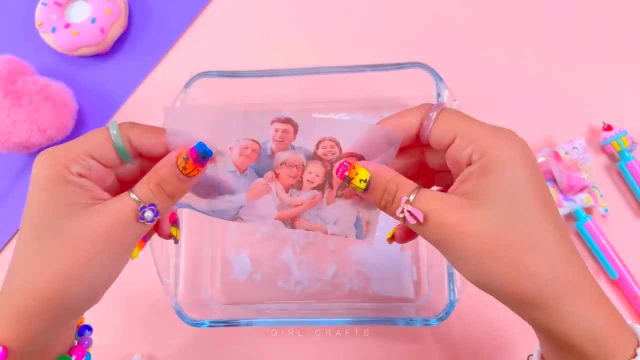 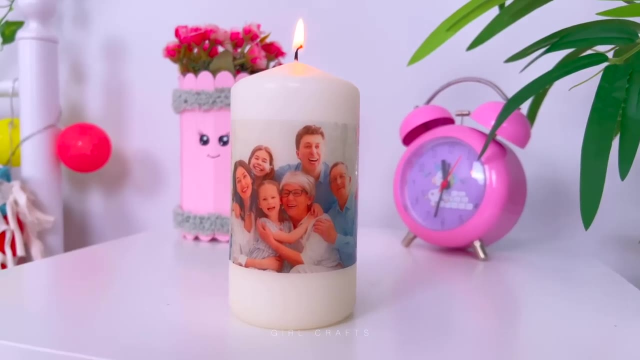 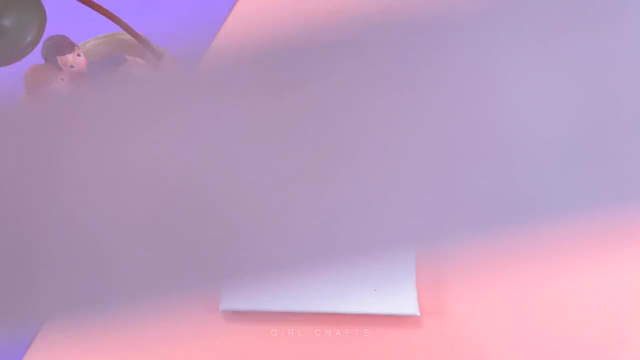 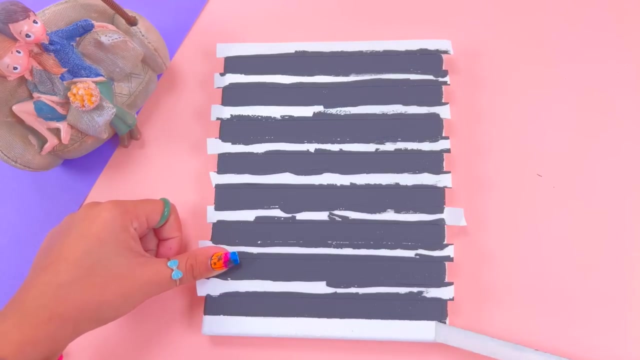 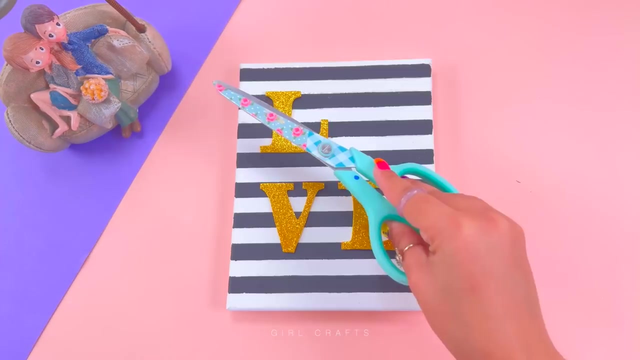 Nobody loves me better. Guess I'm just too scared to settle down. There'd be many nights. I got too high and almost left town. But there's something about you. Something about you. I like About you. I like I get too drunk and too scared and lie to you. 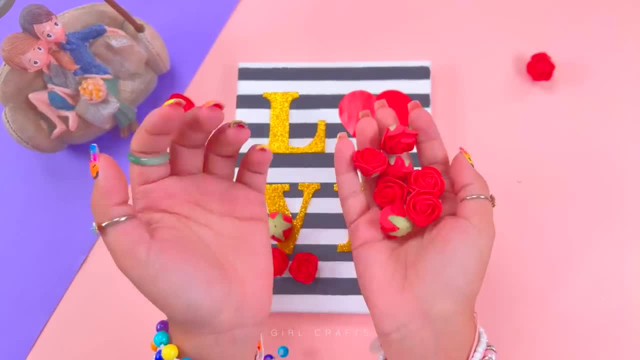 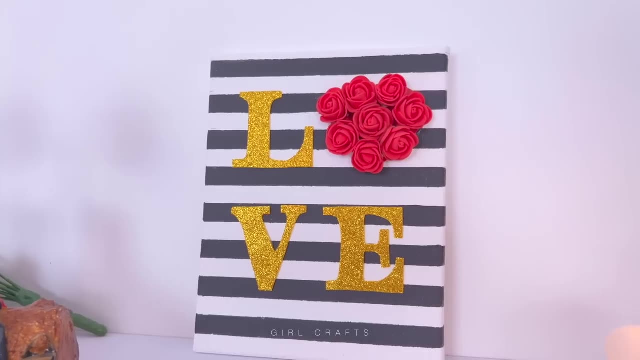 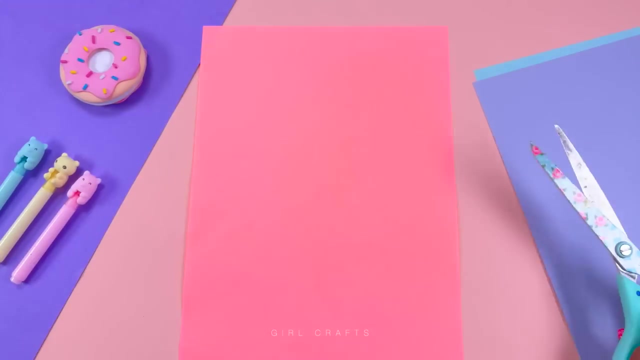 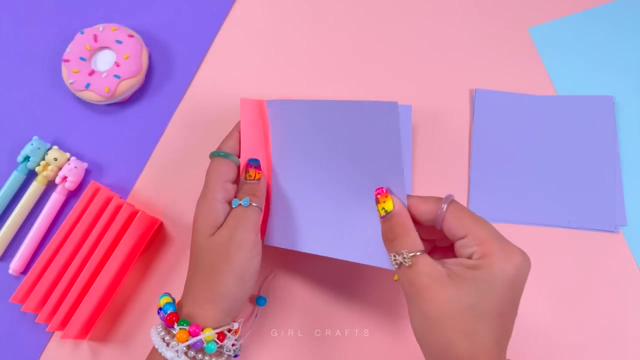 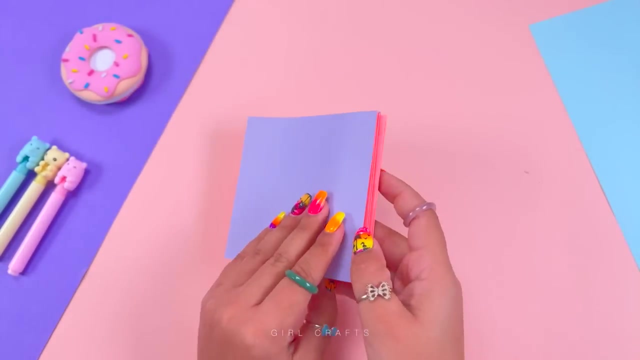 If only you knew I would die for you. One of us, one of us gotta say the obvious. Nobody loves me better. nobody loves me better. I get too drunk and too scared and lie to you. If only you knew I would die for you. One of us, one of us gotta say the obvious. 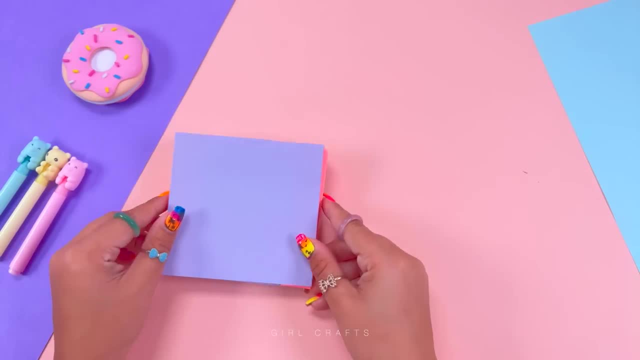 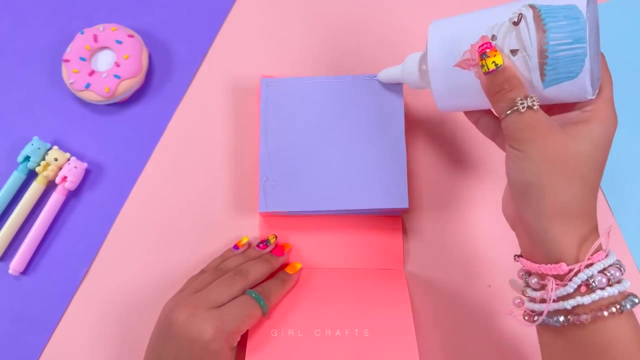 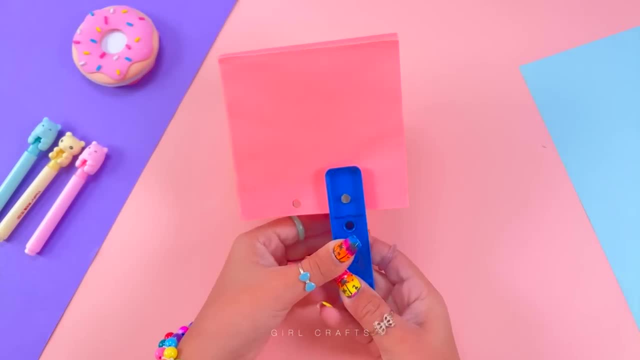 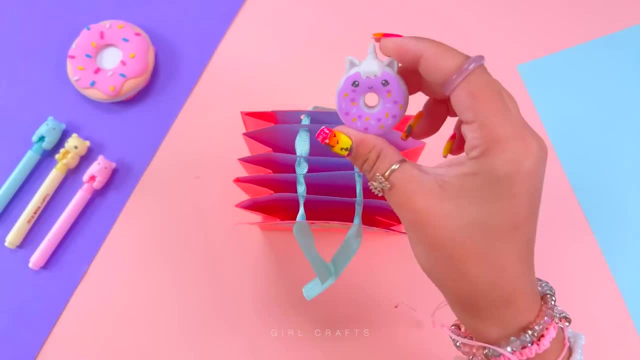 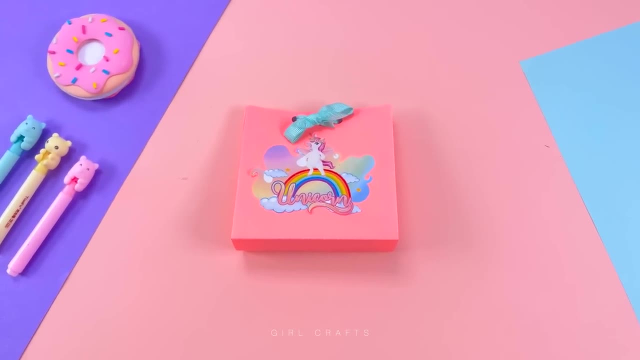 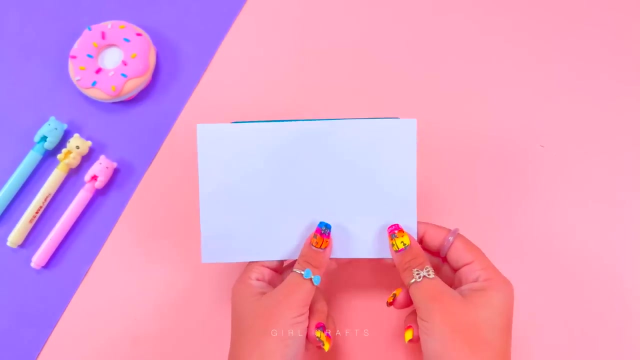 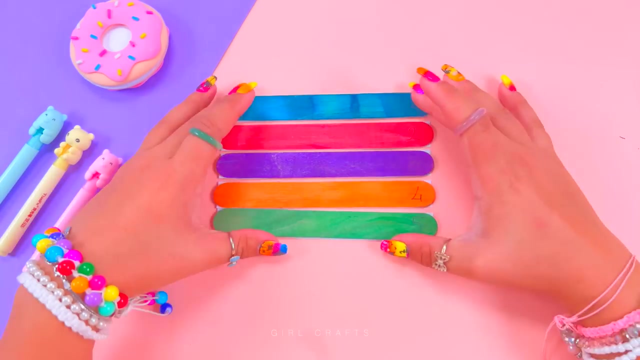 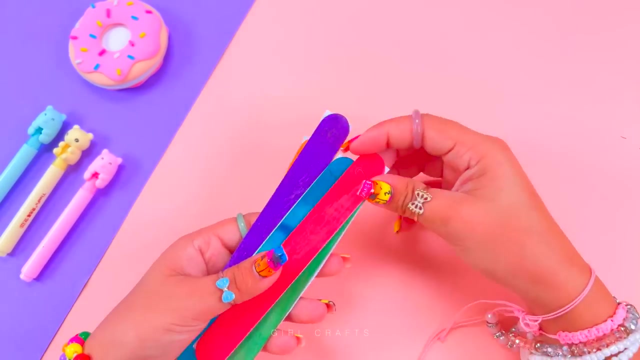 A new place, a new home. For a while, let me feel alive. Nothing to hold me back. Take my time, just enjoy the ride. I know my passing by Life is good, best I've ever felt. Got me up somewhere new, Somewhere I can't find myself. 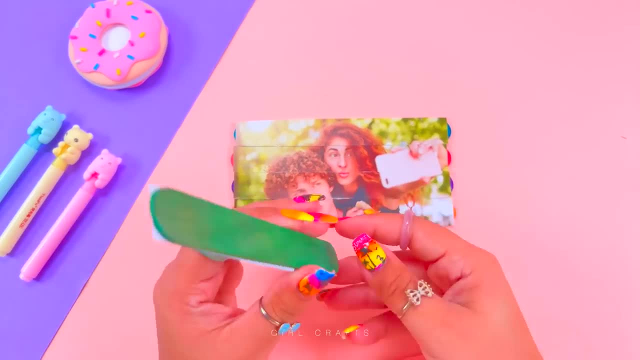 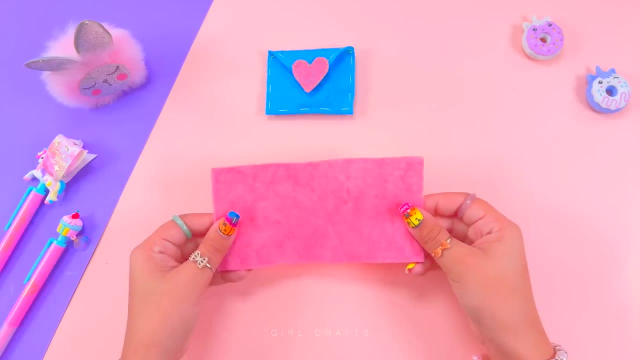 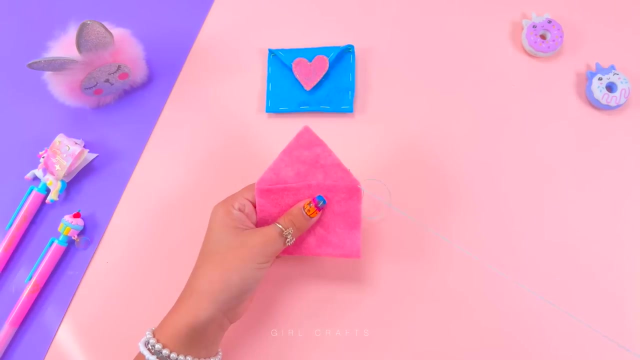 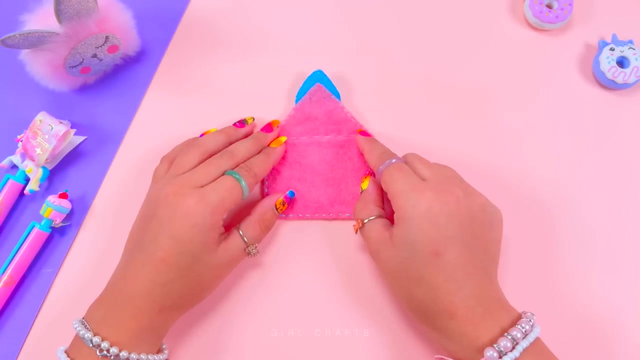